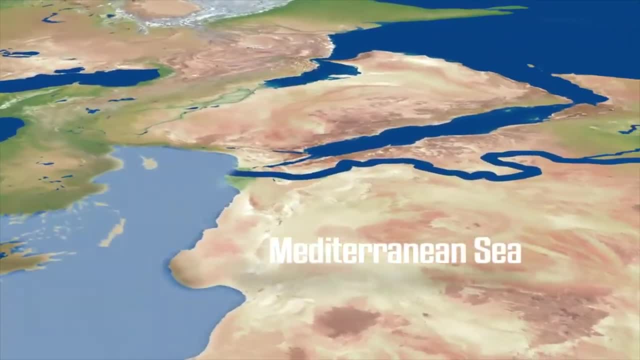 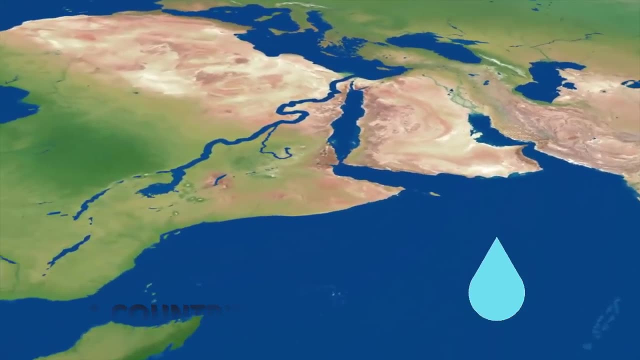 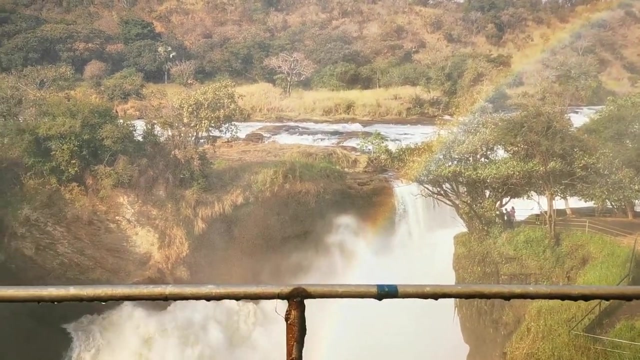 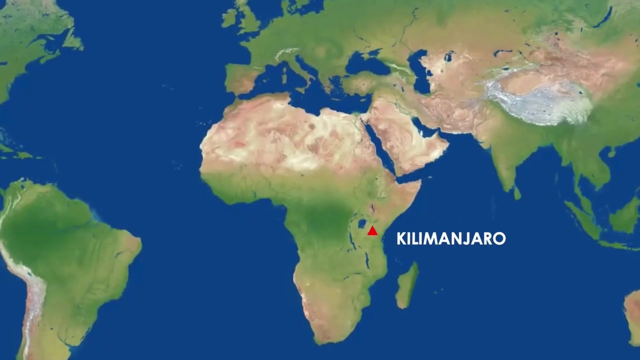 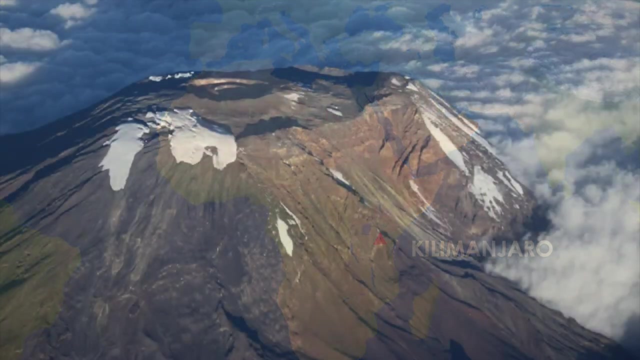 Northward into the Mediterranean Sea. The Nile is very important because it supplies over 11 different African countries with water. Another important fact about Africa is that it has the highest mountain on the continent, the Mount Kilimanjaro. This spectacular mountain is a dormant volcano located in Tanzania. 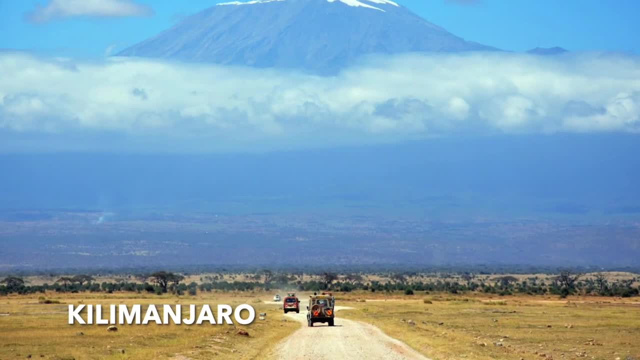 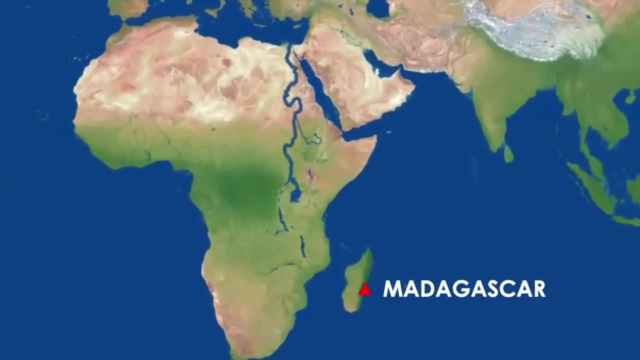 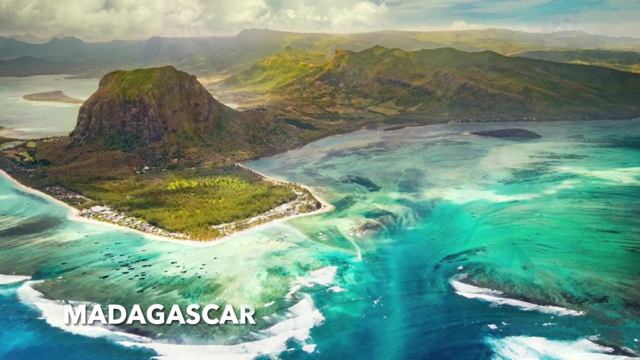 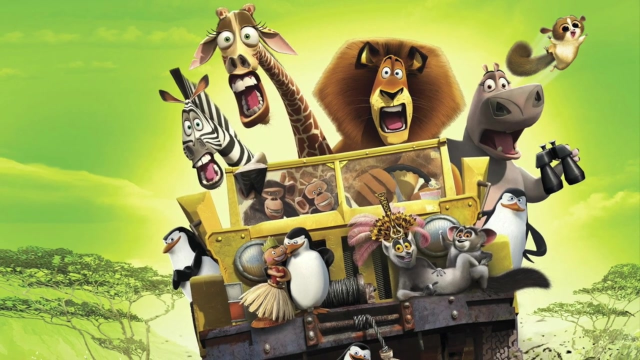 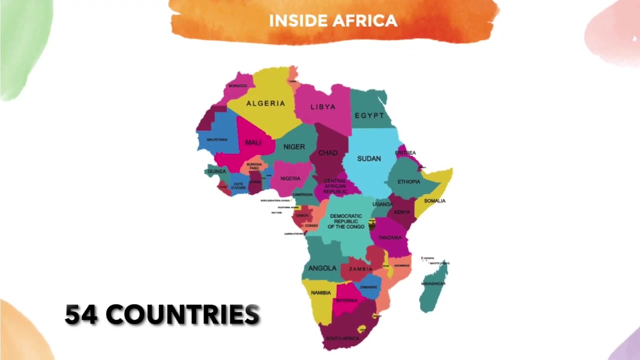 And last but not least, there is Madagascar, Africa's biggest island, located in the Indian Ocean. And, yes, like the movie Madagascar, But it is also very important to know that Africa has 54 countries, more than any of the other continents. 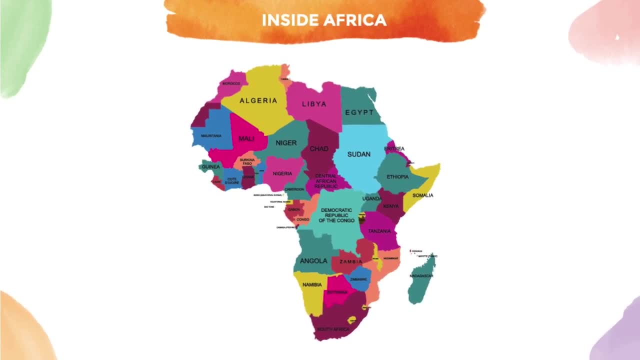 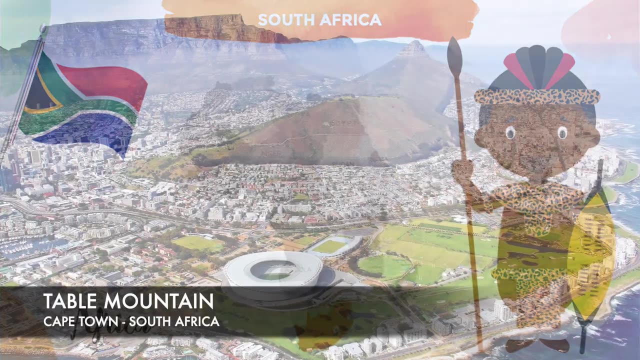 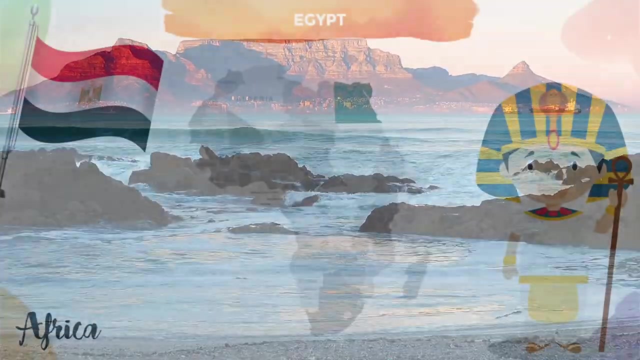 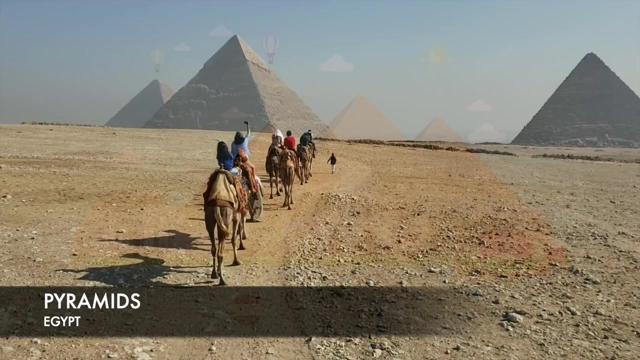 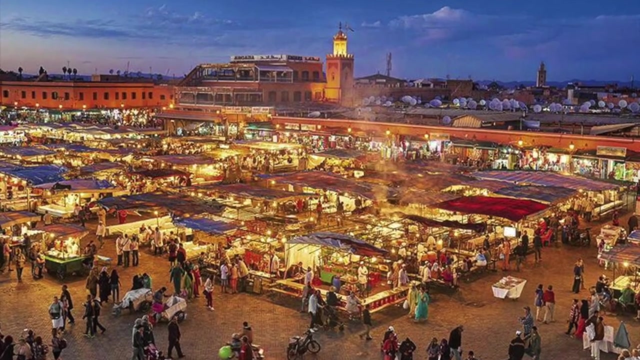 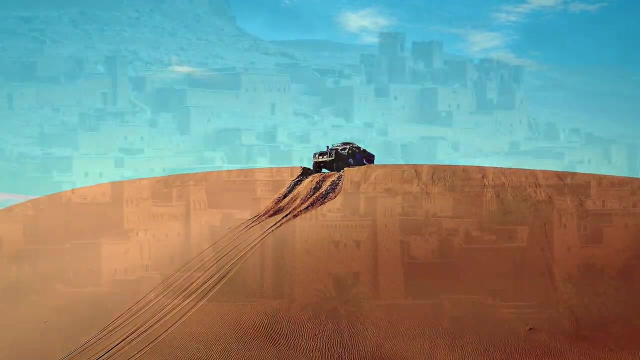 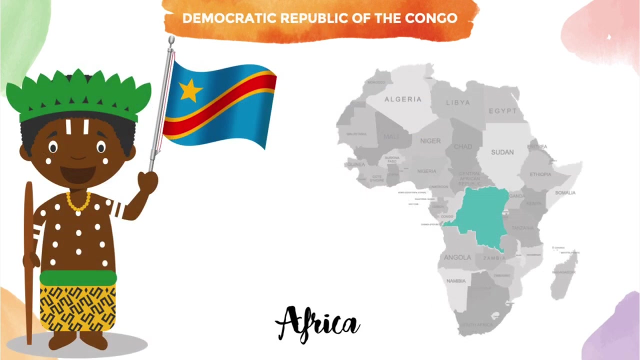 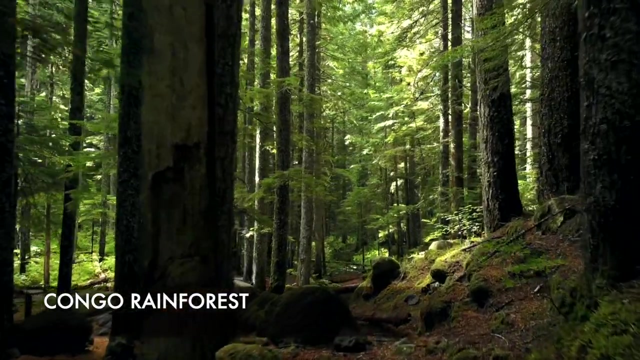 Some of the most important countries inside Africa are: South Africa, where you can find the Table Mountain in Cape Town. Egypt, famous for its pyramids. Morocco, home of markets, Deserts and mountains. Algeria, Democratic Republic of the Congo, where it is part of the famous Congo Rainforest. 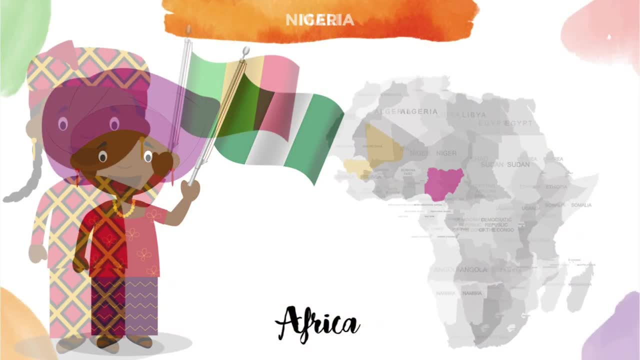 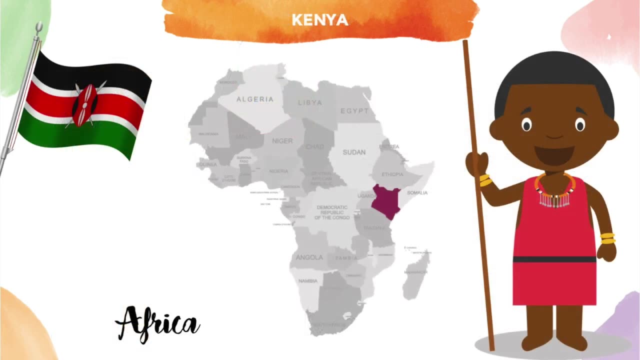 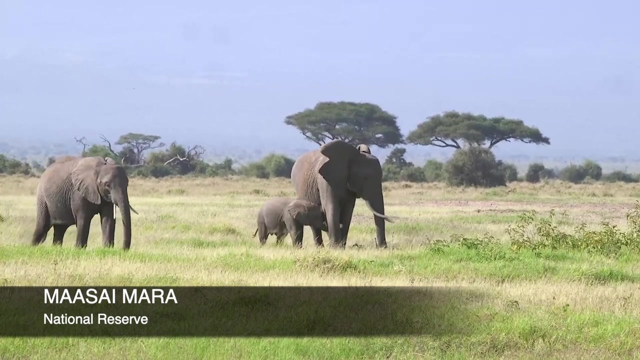 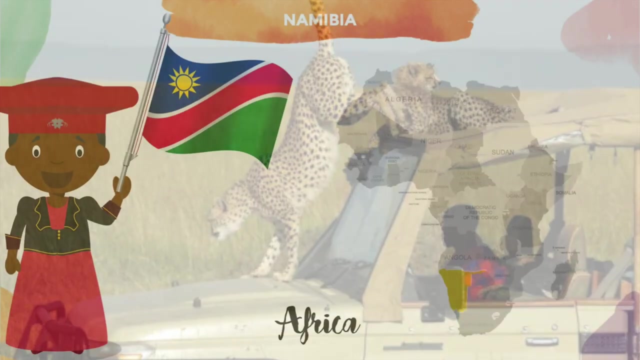 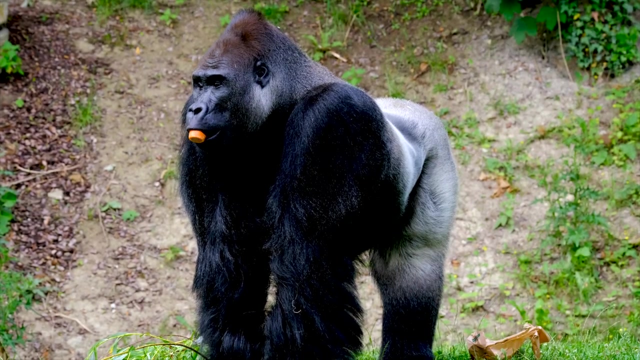 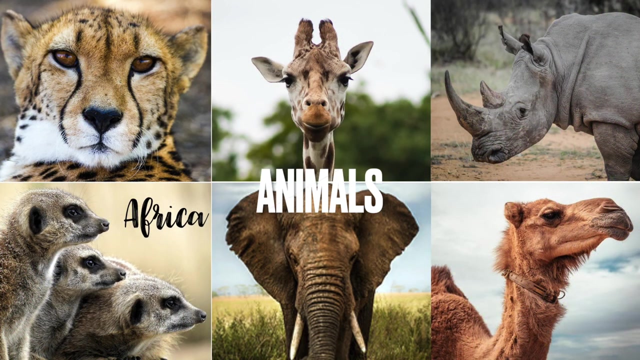 Nigeria, Mali, Ethiopia, Kenya- where you can find the Maasai Mara National Reserve, A very popular safari destination- Namibia And other countries. But when you think about Africa, probably your first thought is, Yes, animals- Africa is home of a variety of animals.